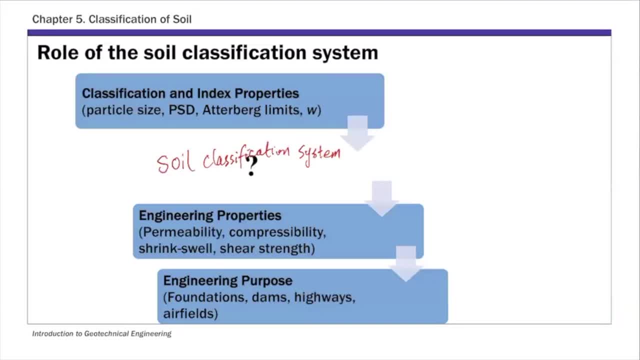 type of soil. I have some idea, some pretty good idea, of what are the probable engineering properties of that soil And again, that properties are what you need for engineering purposes, for design, for construction. So soil classification is really that missing link in that communication language there. And to classify soils we are going to use particle sizes. 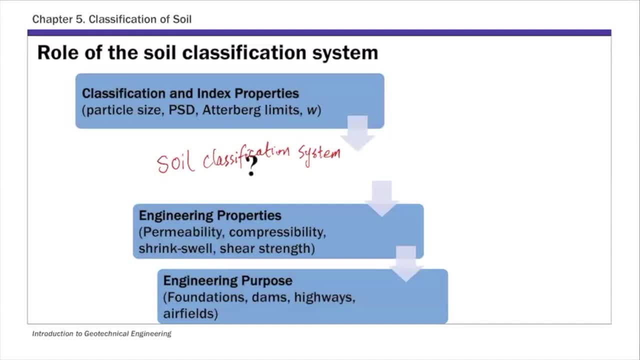 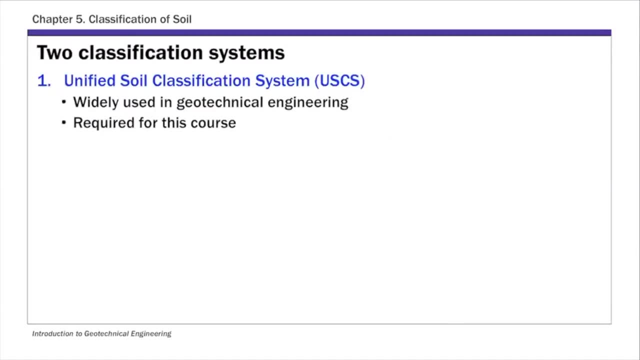 distribution and adipose limits. So we're going to use all these index properties to classify soils. So you are really just telling your students what you need to be doing, which will be your foundation for your class. So here I'm going to go over details of soil. 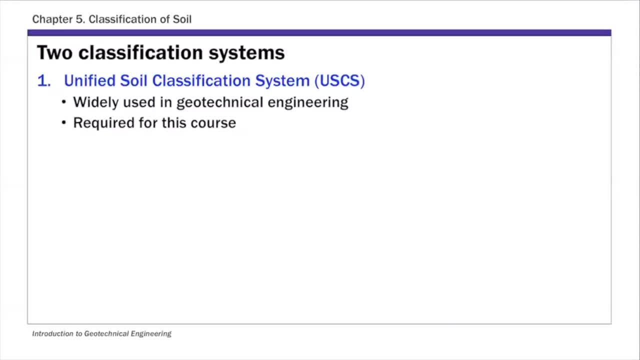 classification systems today And first, there are actually. there are different types of classification systems In this class. we are going to focus on this USCS, or Unified Soil Classification System. So that's what we're going to focus on, because this is the most widely used. 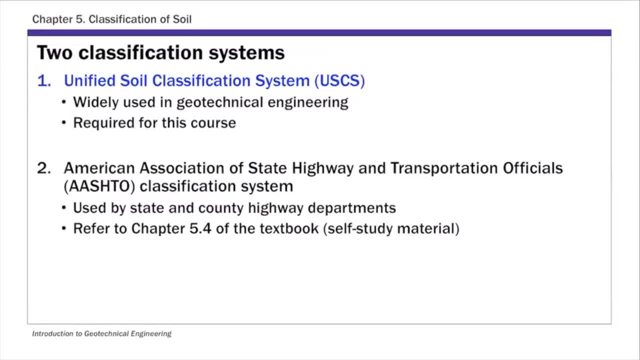 in geotechnical engineering And this is required for this course. And another very commonly used one is this AASHTO system. So this is mainly for state and county highway departments, So they use this system to classify soil for highway systems. 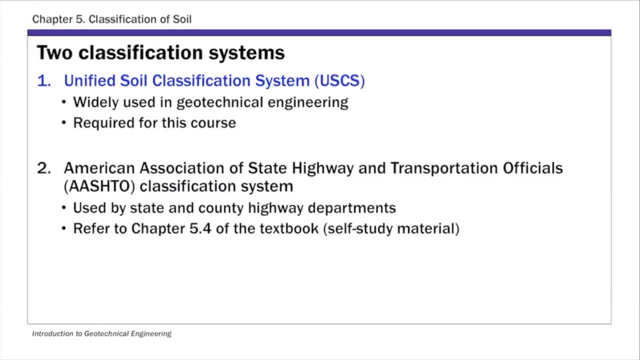 And I've listed here. chapter 5.4 of your textbook actually covers details of this AASHTO system. For both this USCS and AASHTO system, they take into account particle sizes And its distribution And also the edible limits or plasticity of soils. So both systems consider. 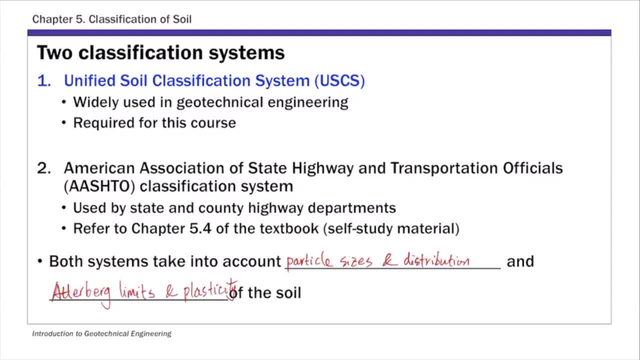 these particle sizes and plasticity of soils. And there are other systems where they only use particle sizes, for instance for classification. But for these two systems they consider both particle sizes and plasticity. And I'm going to go over this unified soil classification. 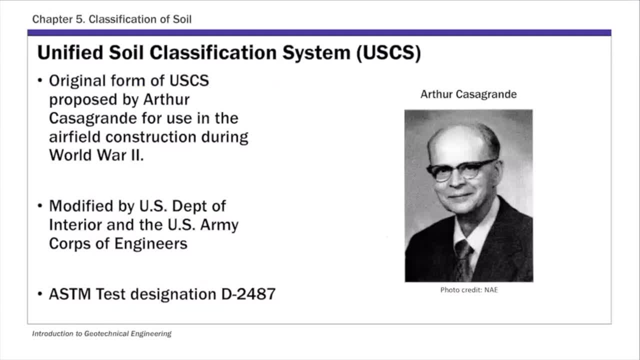 system, USCS, And just a little bit background. This USCS system is the original form of the system is proposed by Arthur Cassegrande. I briefly actually mentioned his name in the last lecture. when we talk 애� cng, when we talk about outward limits, And this is: 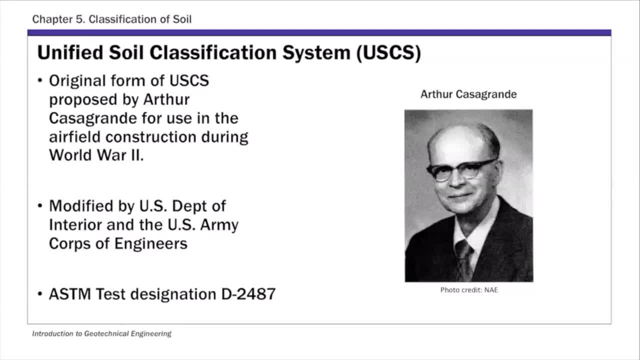 for use in construction of airfield during World War Two, And later that original form is modified by Department of Industries and Industry, So it's made up by um in genau, let's say from calories of nine hundred plus four quadras Metそんなors읍을مَّ요. 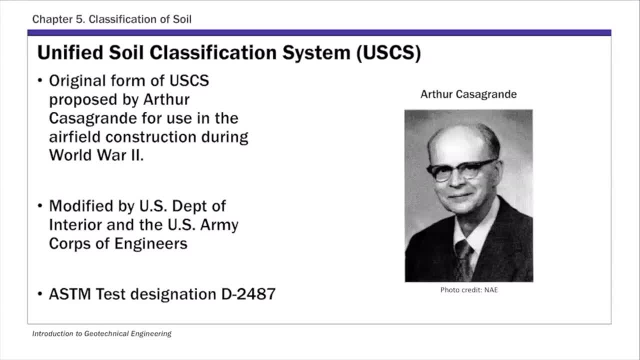 of Interior and US Army Corps of Engineers, and that modified, revised version become ASTM standard, And that's what we're going to discuss today. So I'm going to go over the details of this system and how to use this to classify soils And to use this system. 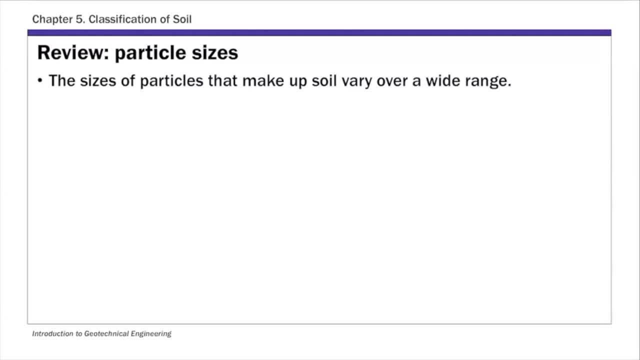 we need a few pieces of information. So just a quick review of what we have discussed so far. First, the particle sizes. So this is chapter two- original soil and particle size, And in chapter two we talked about different types of soils. 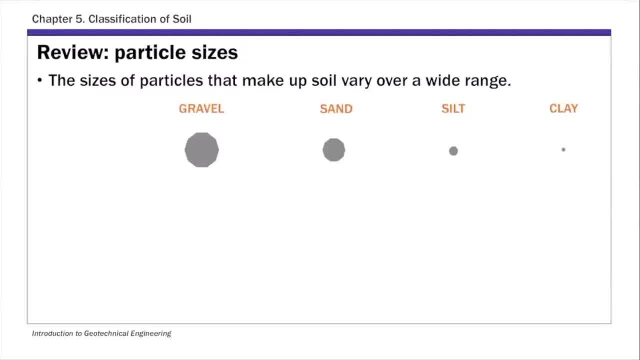 gravels, sands, sills and clay based on their particle sizes And for these two systems, the ASTRO system and USCIS system, and they use different particle sizes to classify soils into gravel, sands and fines, or gravel sands, sills and clay. 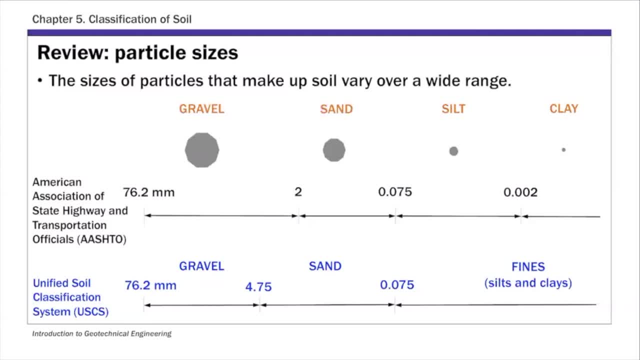 So that's particle size. So they use different particle sizes. And for for again, for our course, this USCIS system, this is required. So for this one there are three key numbers. One is 76.2. 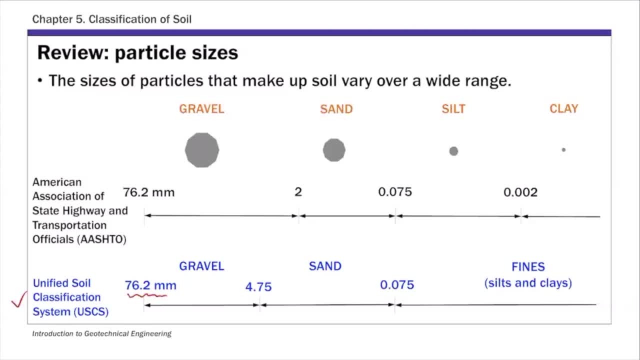 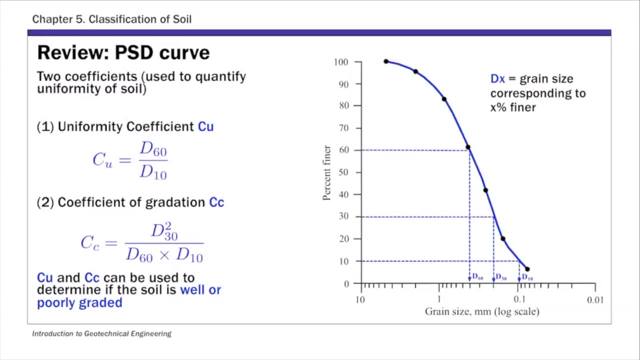 So that's the upper limit of gravel. Four, point seven and five, that's a limit between gravel and sands and then .075 between sands and fines. And the second part is this PSD particle size distribution curve. So recall curve basically showing you the sizes, the particle sizes and its. 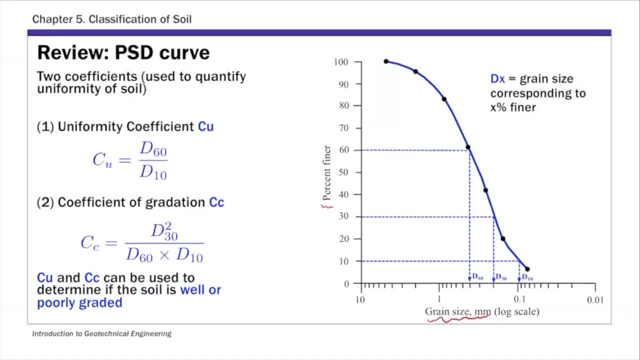 corresponding percentage. So this is a semi-log plot And from particle size distribution curve, what we're going to use for a USCS system are these two indices or these two coefficients. One is called the uniformity coefficient, Cu, and the other one is coefficient of gradation. So specifically, given our PSD, 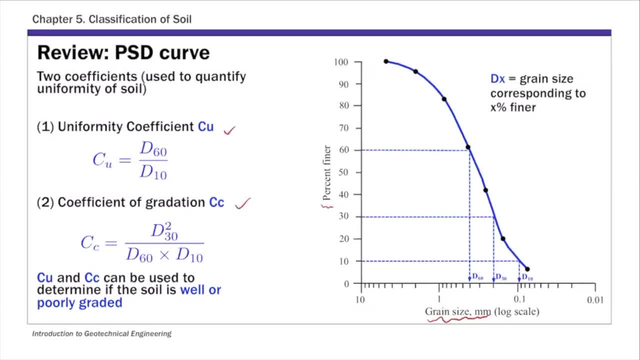 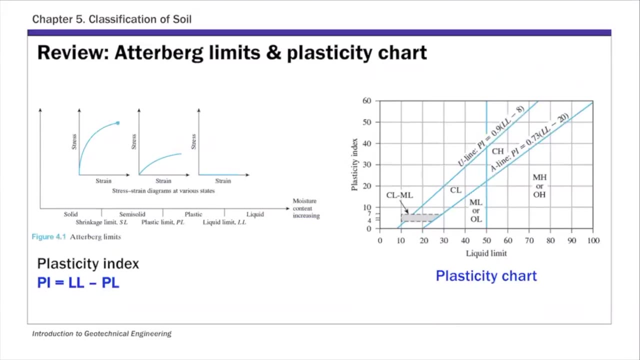 we're going to get these two coefficients and use them when we are trying to classify soils in the USCS system And Cu and Cc they're used for determining the gradation of soil. This is PSD. Just last lecture we concluded chapter 4, so 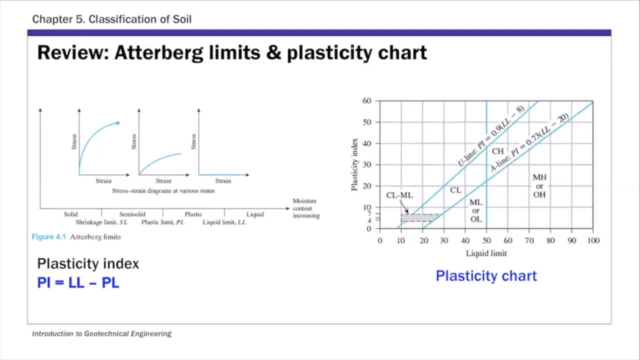 that's on adiabatic limits and plasticity. From adiabatic limits and plasticity, we're going to use this, actually plasticity chart, So something I talked about last lecture in plasticity chart- remember it's liquid limit versus plastic index chart- And we're going to 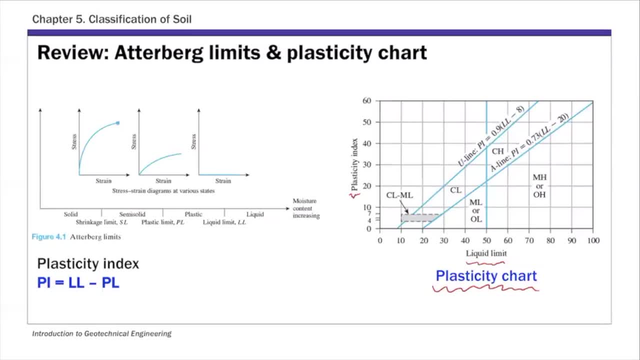 use this chart to help us determine if the fine contents are sills or clays In plastic index, just to review it's difference between liquid limit and plastic limit here. Alright, so that's a very quick review, and then I'll see you at the next class. 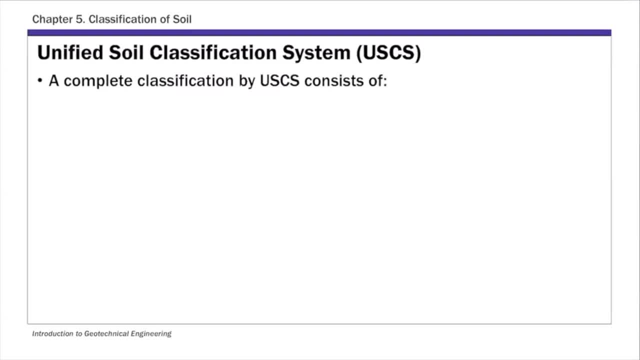 Then I'm going to introduce this USCIS system in details. So in the USCIS system a complete classification has two components. So the first one. so I'll start with group symbol action. The first one is group symbol And the second part of the USCIS system is the group name. 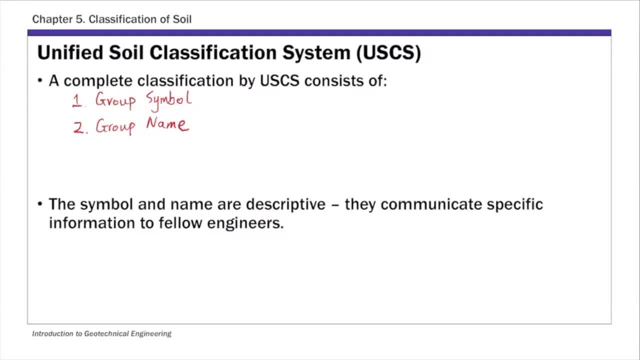 And this is a difference between the USCIS and AASHTO system. So in the USCIS system the group symbol and group name, they are descriptive, So meaning they communicate specific information. If you look at the group symbol and group name. 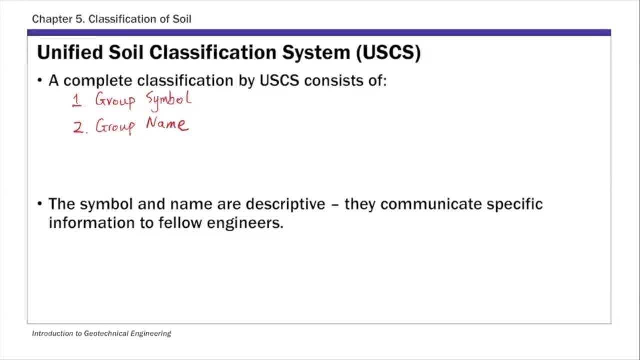 you can immediately tell what kind of soil it is. The AASHTO system, on the other hand, uses just letters and numbers. So the names in AASHTO system? they are not descriptive, So you need to refer to a table. 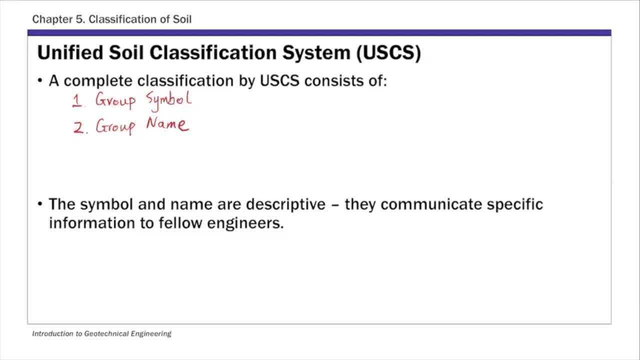 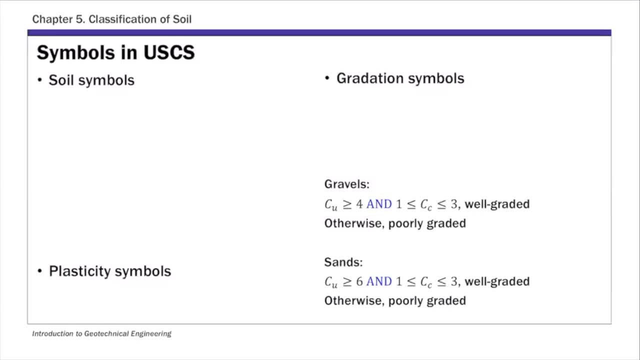 to really get the meaning of what A1 is, A2 is, A3 is Okay For USCIS. so the first thing I want to go over is those symbols in USCIS, So the first part of the member of the USCIS system. 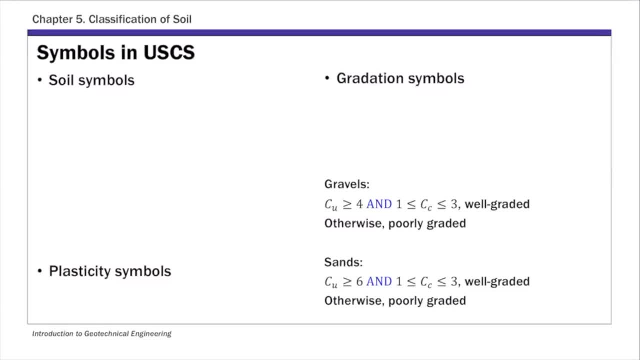 is group symbol, And there are a number of symbols in the USCIS system And I classify them into soil symbols, plasticity symbols and gradation symbols. I'm going to go over all of them. The first one, soil symbols. 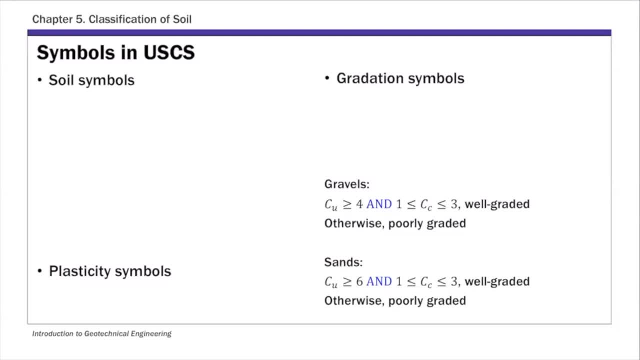 There are six soil symbols. Start with the first one. So the first soil symbol is: G stands for gravel, And second one, S. this stands for sand, And then M stands for silt And C for clay. Again, as I mentioned, those are descriptive names. 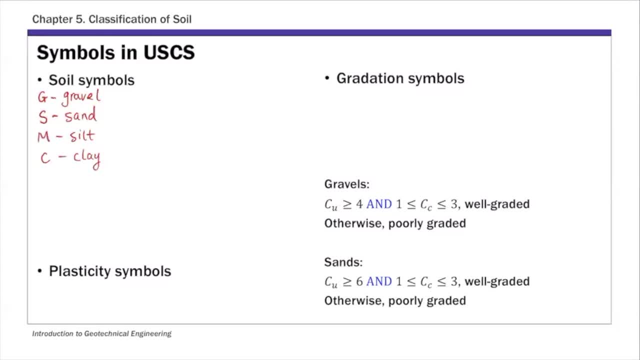 You'll see letter G. you can immediately link that, relate that to gravel. And the other remaining two are O for organic silt and clays, And last one is P, small letter T, And this is for peat, muck and highly organic soil. 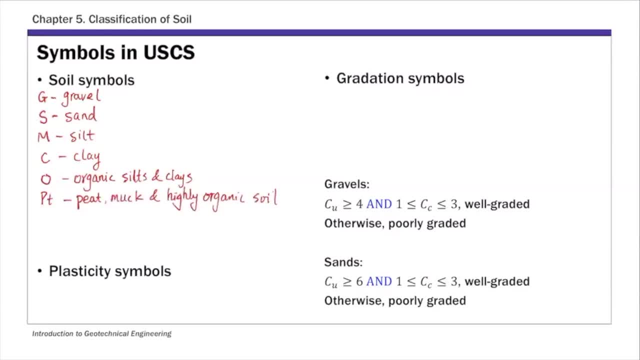 So that's the first group of symbols- soil symbols, And these are very, very descriptive. So you see the letter, you can immediately link that to a particular soil. And the second group is plasticity symbols, And there are two letters for plasticity symbols. 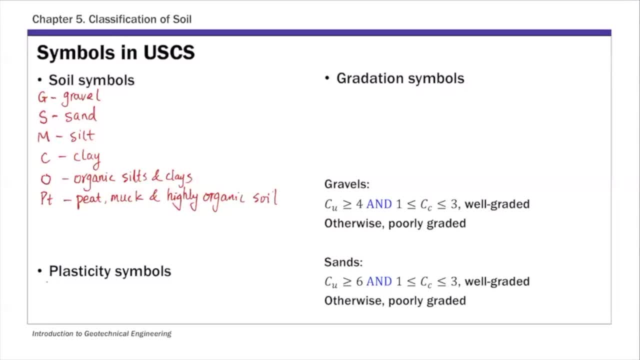 First one is L for low plasticity And second one is H for high plasticity, That's plasticity symbols. And the third group are gradation symbols And gradation symbols also, there are two: W for well graded and P for polygraded. 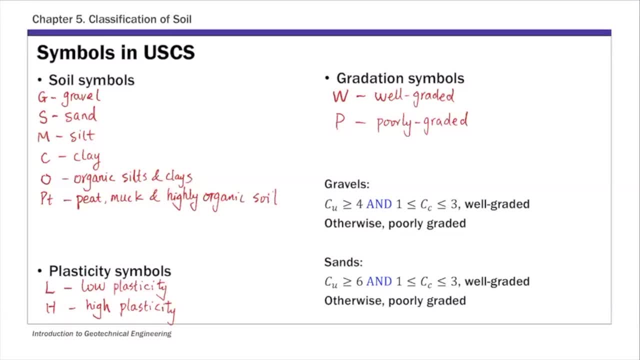 So those are two, O and P. those are all the symbols in the USCS system. And for gradations, remember there's something we cover in chapter two and you can use Cu and Cc to determine if soils are well or poorly graded, For gravels, for instance. Cu. 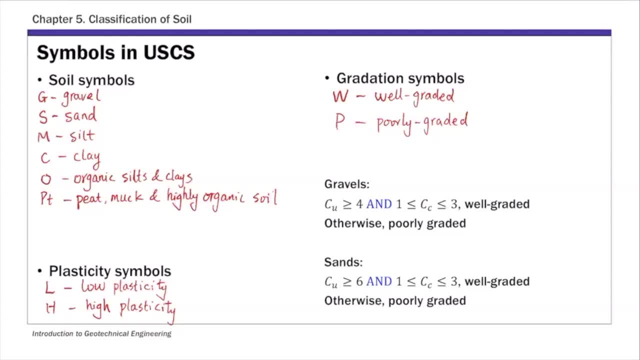 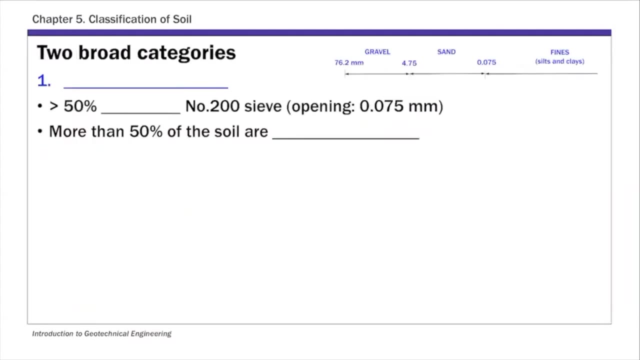 greater than 4 and Cc between 1 and 3 are the conditions for well graded soil And for sands. Cu greater than 6 and Cc between 1 and 3 are conditions for well graded soil. So that's symbols in the USCS system And next in the USCS system. 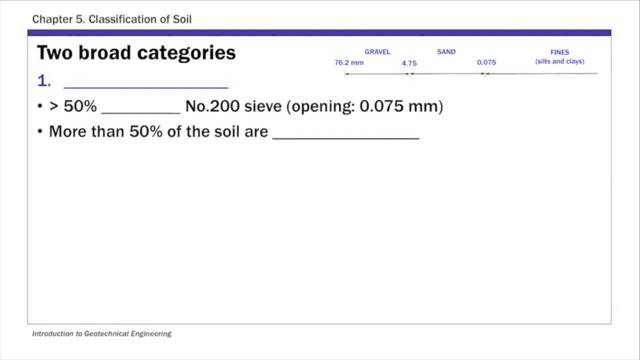 soils are put into two broad categories based on the percentage of fines and coarse-grained soils. So the first category is called coarse-grained soil, And for coarse-grained soils more than 50% of the particles are retained on or above Cc. 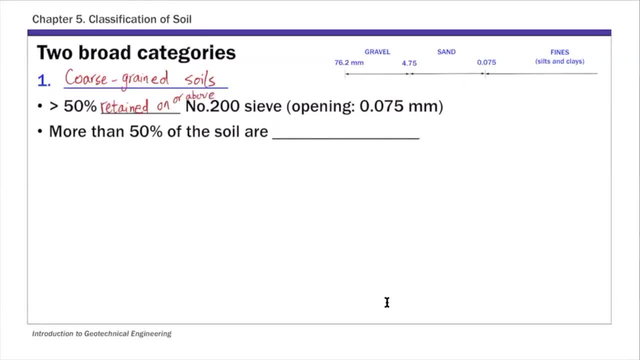 number 200, seed, And this simply means more than 50% of the soils are gravels and sands. So that's the first broad category: coarse-grained soils. More than 50% are gravels and sands. The second category is fine-grained soils. For fine-grained soils, this means less than 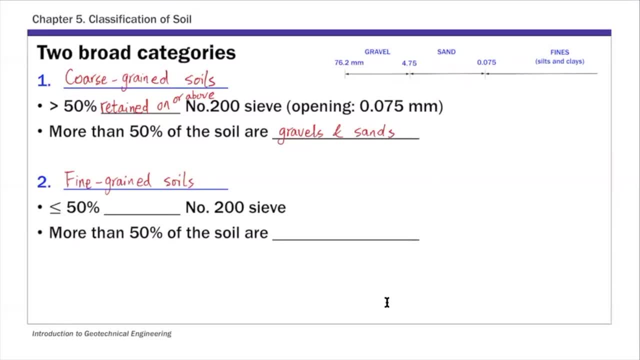 or equal to 50% of the soil they retained. Okay, so let me actually write it this way. So I'm going to modify this size slightly. Okay, So I'm going to write using larger than or equal to, So for fine-grained soils, more. 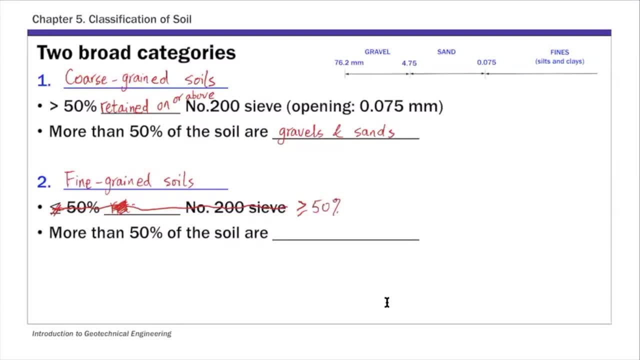 than 50%. they pass number 200 seed And that means more than 50% of the soils are fines, which includes silt and clays. And those are the two broad categories. There's actually another one, that's highly organic soils. 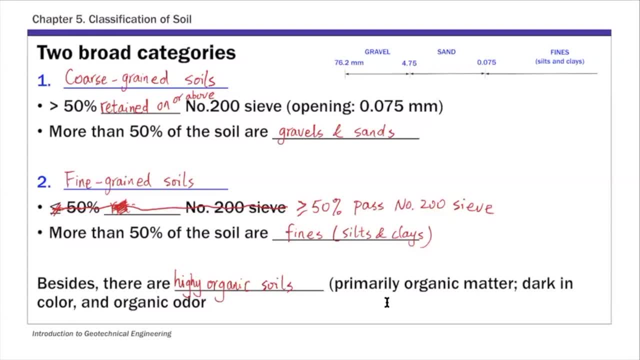 Highly organic soils are characterized by basically dark green color and organic odor And, for this course, unless it's explicitly given, we're going to assume all the soils are inorganic And that's where we're going to use particle sizes and adverb limits to classify the soil. 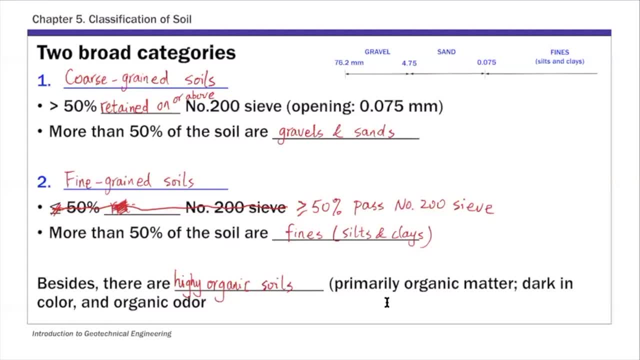 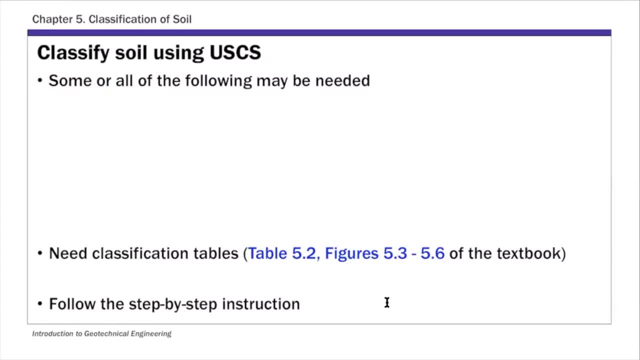 Okay, So for so these are the two broad categories. So then, to classify a soil using USCIS, first you need some information about the soil. So basically, those are the index properties. So we need the following information: The first one is from sieve analysis. 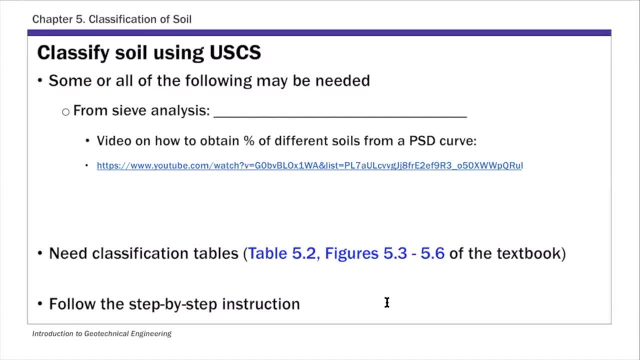 You need the percentage of different types of soil, Percentage of gravel, Percent of sand, Percent of fines, Cu and Cc. So, again, you need some or all of the following information And for how to obtain these different types of soil, the percentage of different soils from a PSD. 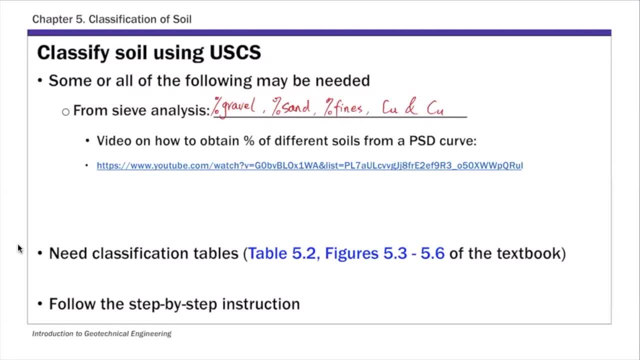 So this video- this is on our YouTube channel. This is a PSD curve basic video And that covers how you obtain this information If you, if you're given a PSD, And then from adverb limits, something we discussed last week. 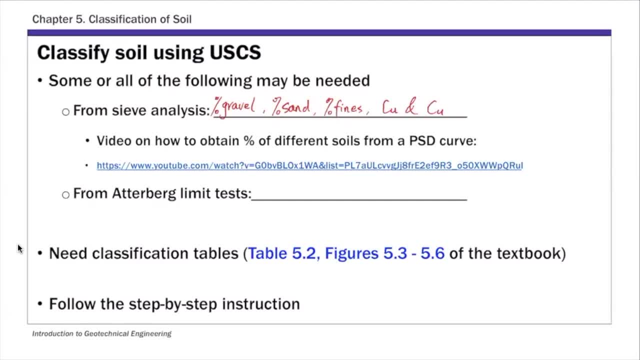 This is, you need liquid limit and plastic index, Which is defined as LL minus PL. So you need these pieces of information And then, to once you have this, this information, then you need classification tables For our textbook, table 5.2. 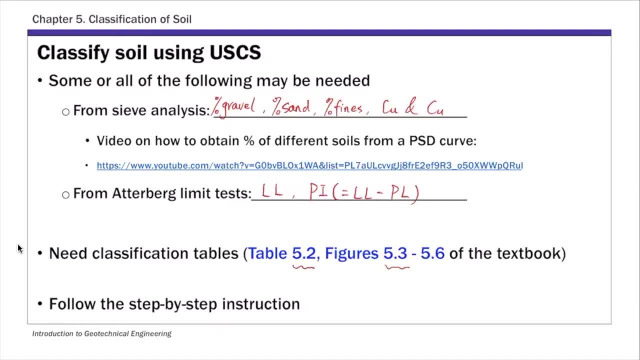 Figures 5.3 to 5.6 are the classification tables. you need to determine group symbol and group name. And then the next are just some step-by-step instructions. So I'm going to go over these instructions, But before that let me show you what these tables look like. 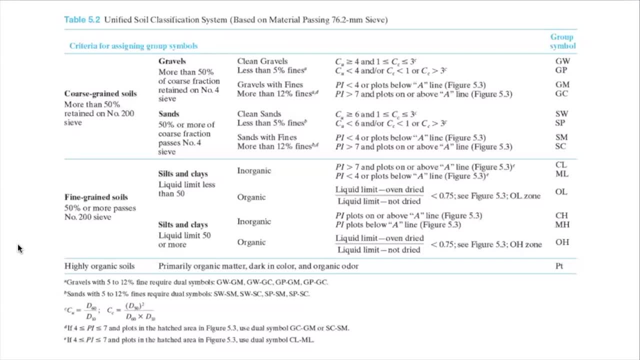 The first one. this is table 5.2.. This is the main table to obtain group symbol And I'll come back to this in just a little bit. I'll explain all these details, all the details here. So this is table 5.2.. 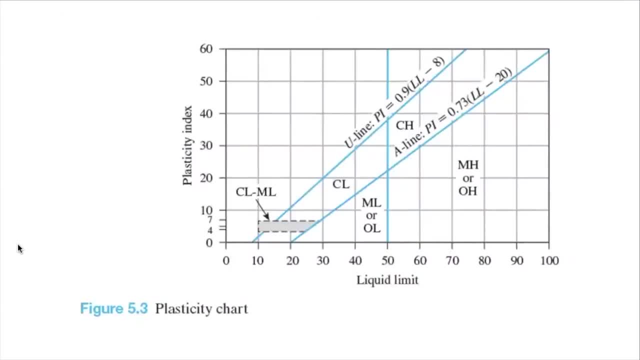 Figure 5.3 is that plasticity chart? So that's what you use to determine the fine contents, to tell if they are silts or clays. And then 5.4 to 5.6, these three figures are group names. 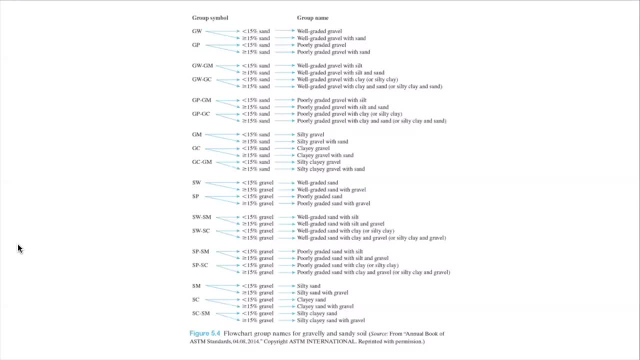 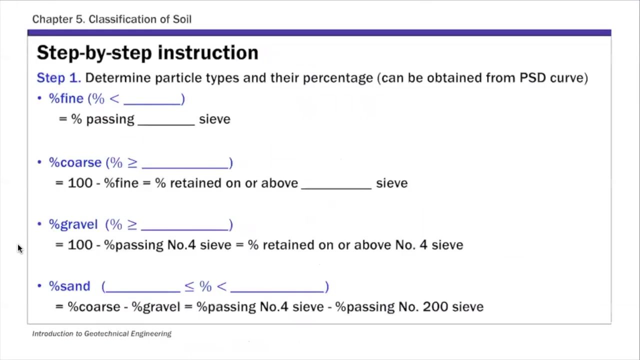 So remember, USCIS system consists of group symbol and group name. So 5.4 to 5.6, these figures are used to determine group names. Now to this step-by-step instruction. So I'm going to go over this in detail with you. 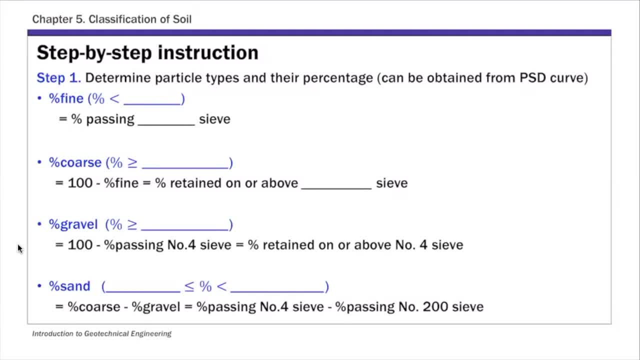 And we're going to go over at least one example today For step-by-step instruction. the first step is to determine particle types and their percentage. So basically these are from C, So this is a C-shape analysis, It's like. so there are two scenarios basically. 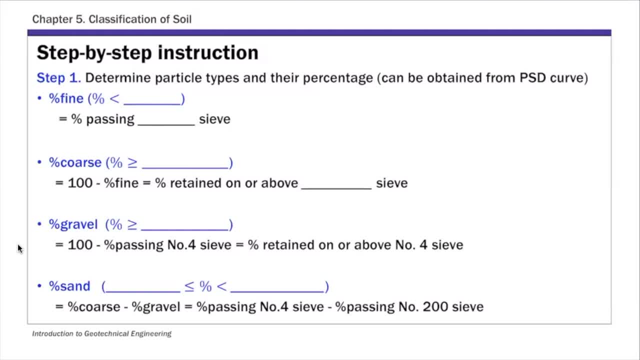 One is you're given a PSD curve And then you obtain these percentages directly from the PSD curve. So that's one scenario. The other scenario is you are given basically the sieve analysis data directly, So you're given the percentage passing for a specific sieve number. 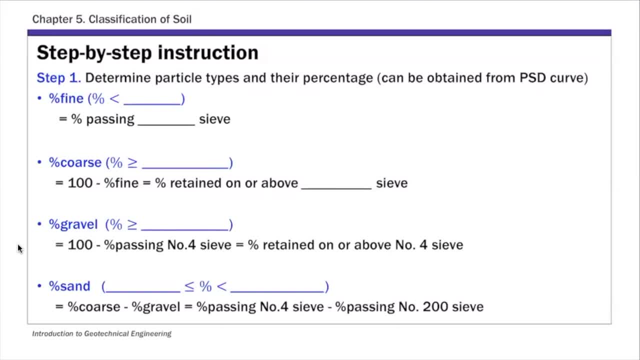 And you can also get these percentages from that table as well. Okay, So we have homework problems or examples for both types And for percentage of fine. so it's percentage smaller than 0.075 millimeter. Okay, So if you are given PSD curve, you can get the percentage finer than 0.075 millimeter from a PSD curve. 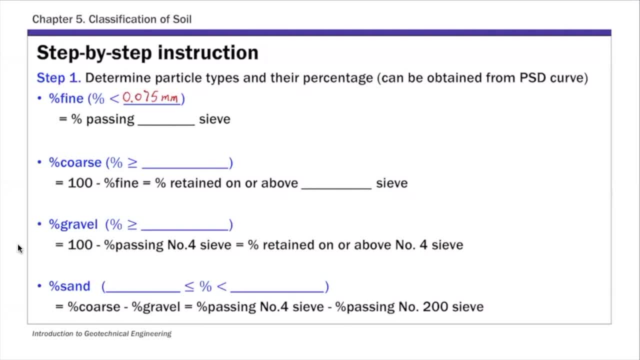 And if you are given the raw data of sieve analysis, then percentage of fine is basically the percentage passing number 200 sieve And then percentage of coarse. this is percentage larger than 0.075.. And this is percentage of soil retained on or above number 200 sieve. 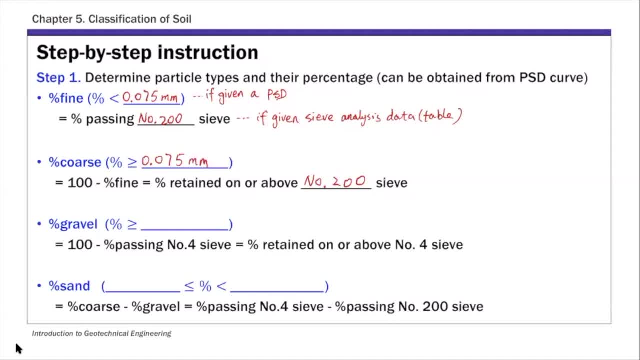 Then percentage of gravel, and that's percentage greater than 4.75 millimeter, And this is basically that number four sieve size. So it's a percent retained on number 200 sieve. That's percent of gravel And then sand. 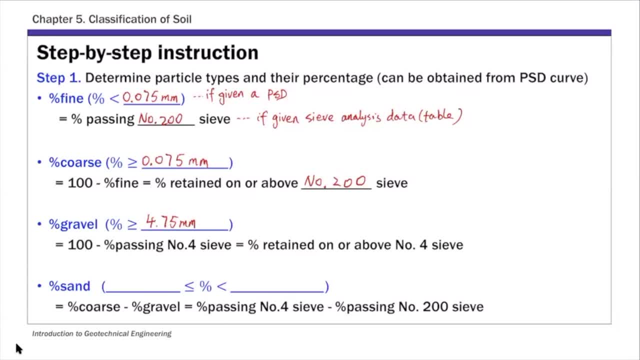 so it's percent between 0.075 and 4.75.. So that's the percent of soil in between these two numbers, these two sizes, And it's basically, if you have percent of gravel and percent of coarse, calculated, it's a difference between these two. 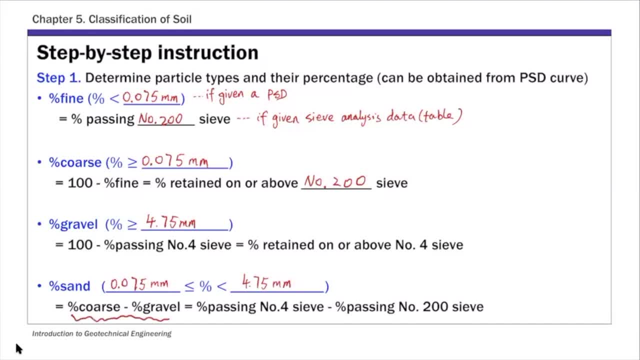 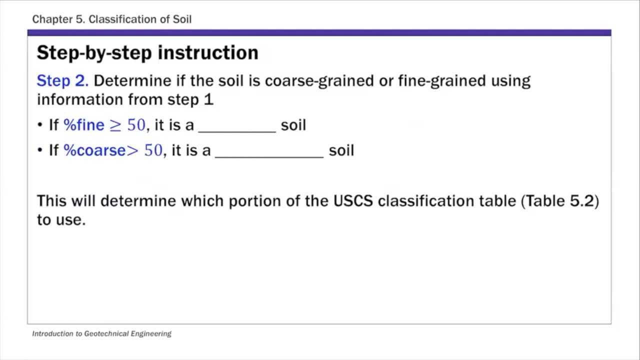 So that's a percent of sand. So that's the first step, basically getting all these percentage of different types of soils. And second, once you have that information, is to determine if soil is fine or coarse-grained. So if 5% greater than 50%. 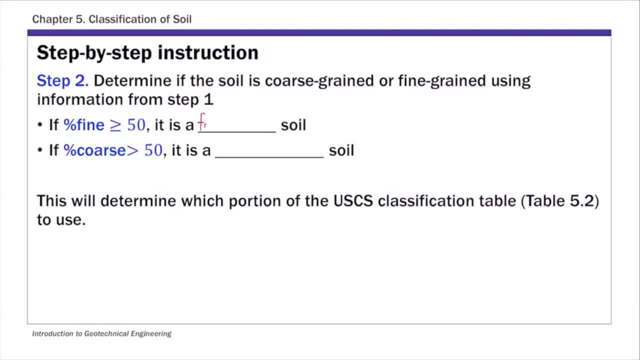 that's a fine-grained soil. And if you have more than 50%, if you have more than 50% of the soil being coarse, that's coarse-grained soil. And remember, these are the two broad categories in the USCIS system. 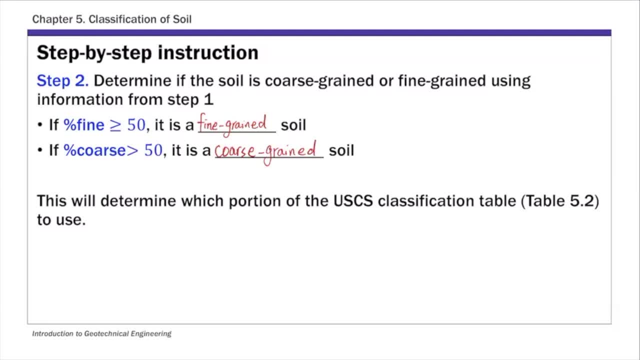 fine-grained and coarse-grained soils And this will determine which portion of that table- 5.2, you need to use to get the group symbol. Again, I'm going to go over details on that table. This is step two. 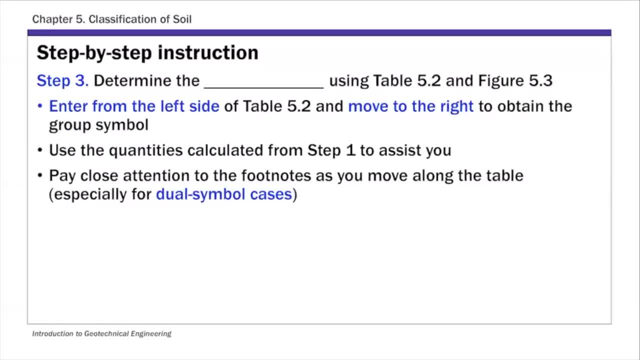 And then step three, using that table 5.2, and also along with that plasticity chart. So we're going to find the, find out the group symbol. So determine the group symbol first, And to do that so we're going to enter from the left side of table 5.2,. 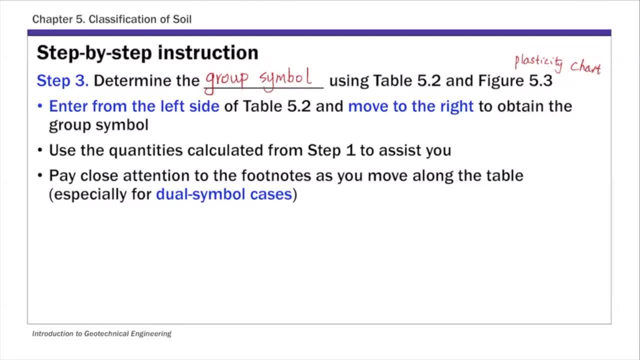 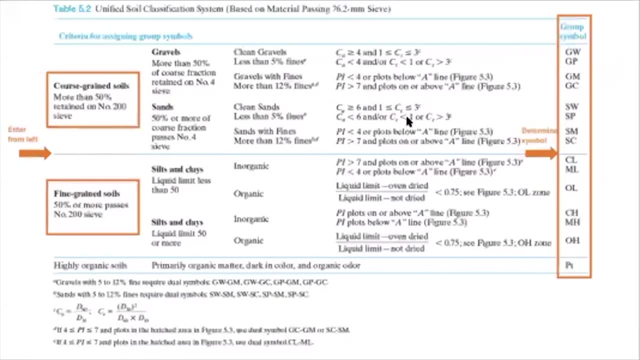 and then use the information you calculated from one to two to determine the, to move to the right, basically to find the group symbol. Let me show you what this table looks like. So this is that, table 5.2.. And in this table, 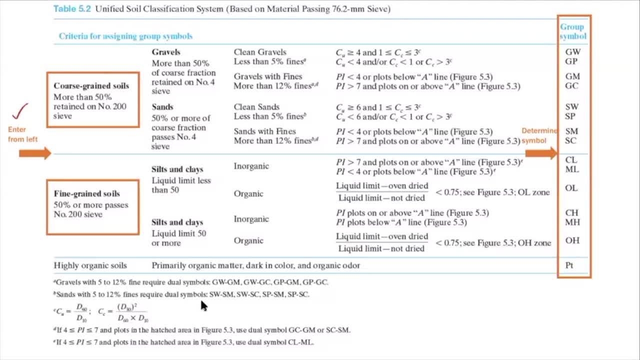 as I mentioned, you enter from the left And if you enter from the left you will see there are two broad categories- that coarse-grained soil and that fine-grained soils- And then you move basically to the right-hand side using the information you calculated from step one to two. 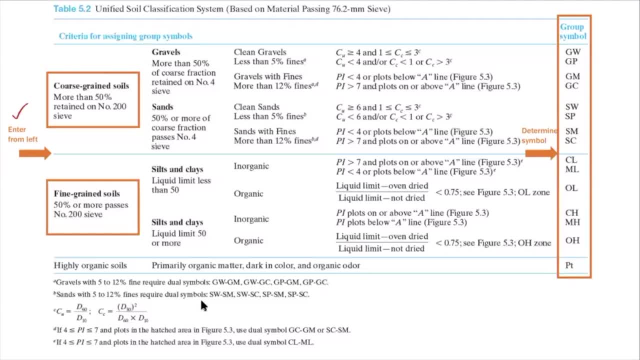 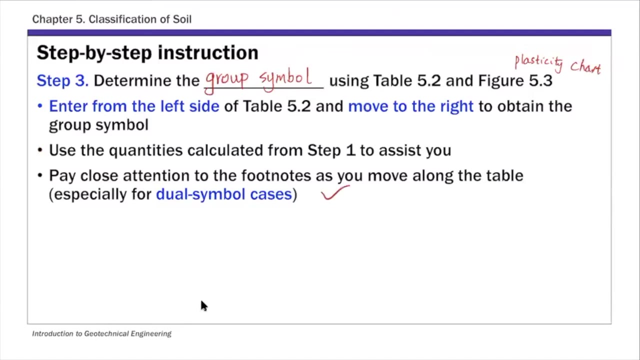 Eventually you're going to exit on the right-hand side and find the group symbol. So that's what you get from table 5.2- group symbol, And so I put a note here. As you move along the table, you need to pay special attention to the dual symbol cases. 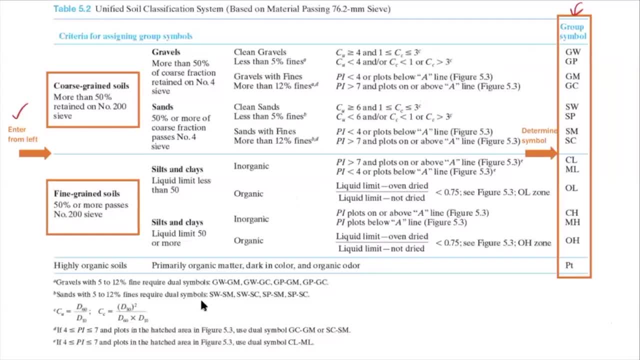 So these footnotes basically. So, if you look at these footnotes, so these footnotes are for dual symbol cases, And that's that's particularly challenging for for this classification system, these dual symbol cases, And that's where I find many students struggle. 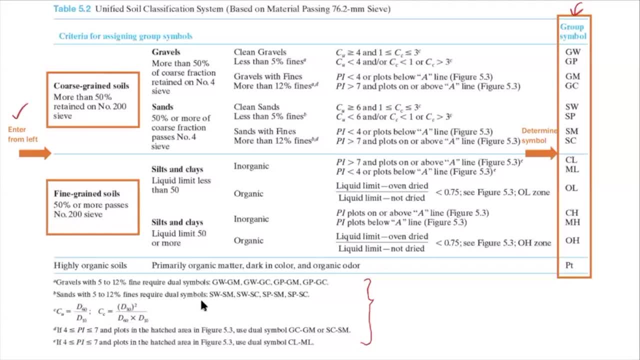 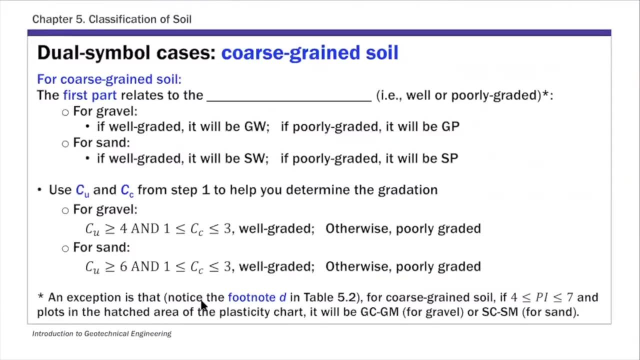 with this UI system is dealing with these dual symbol cases, So I created additional instructions. Okay, So, dual symbol cases. So this is a little bit tricky. I'm going to go over dual symbol cases for coarse-grained and fine-grained soils. 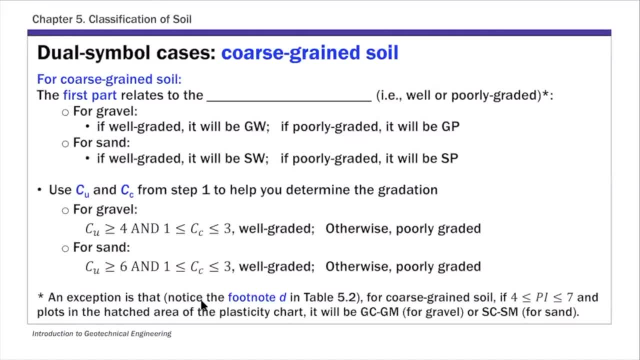 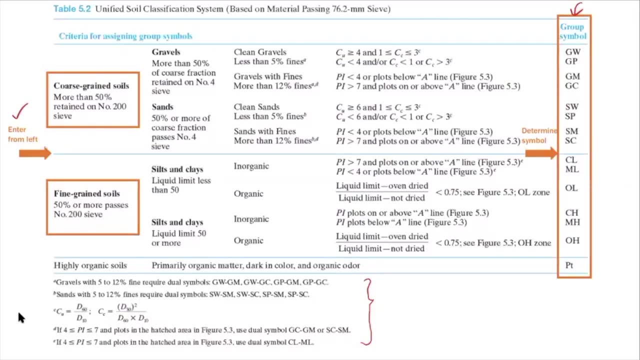 So they are slightly different. For coarse-grained soils the dual symbol cases are, let's say, for: the first part of the dual symbol relates to the gradational soil. So let me show you one example. So look at this first footnote A here. 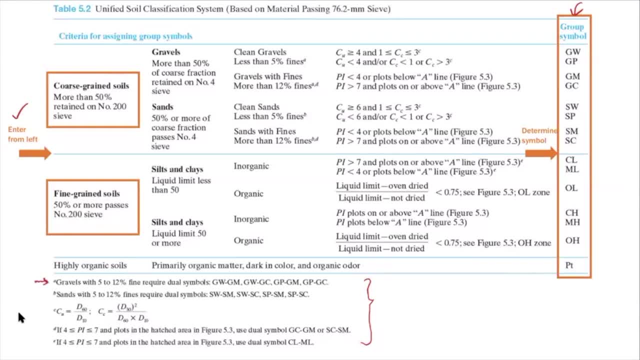 Footnote A. you see, all these are dual symbol cases And you'll notice that the first part of the dual symbol is either GW or GP. So that means it's either well graded gravel or poorly graded gravel. So the first part of the dual symbol relates: 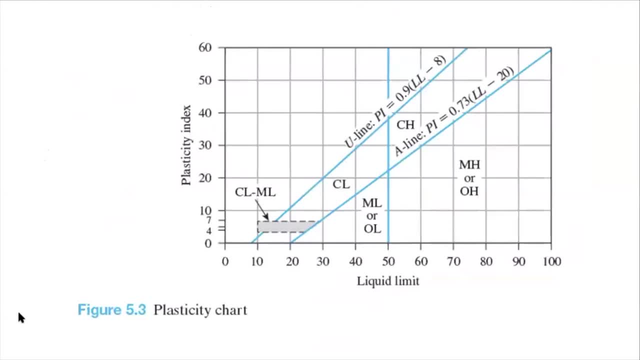 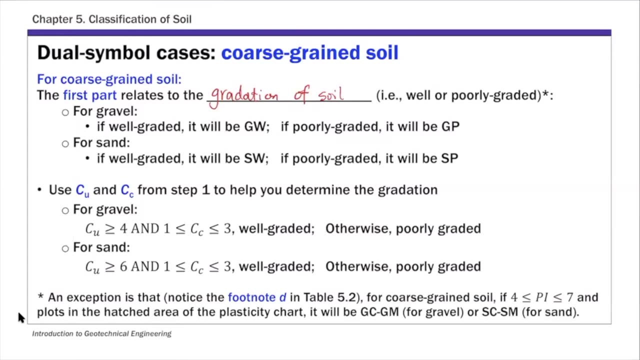 to the gradation And to determine that you need CU and CC. So that's what's shown here. So you use CU and CC to tell you if the gravel or the sand are well or poorly graded. So that gives you the first part of the. 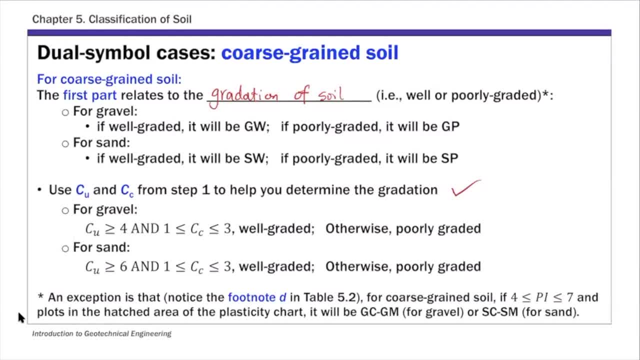 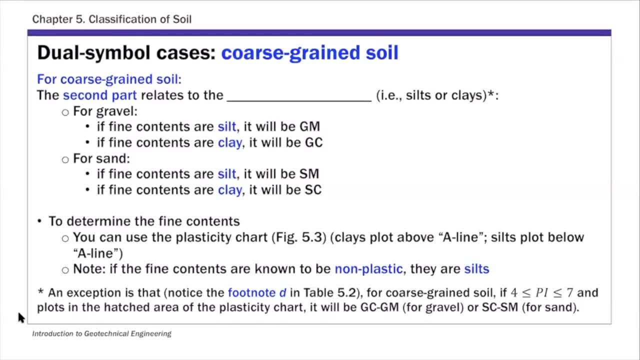 dual symbol, And the second part of the dual symbol for coarse-grained soil relates to the plasticity or the fine contents, As shown here. if fine contents are sealed, it will be M, And if fine contents are clay, it will be C. 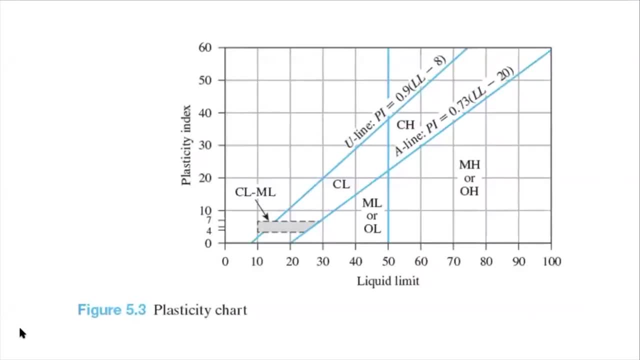 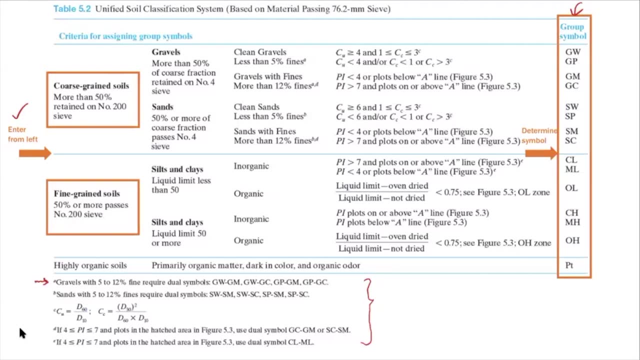 So again, let's look at that table. Let's use this footnote A here. So footnote A, as I mentioned, first part relates to gradation: It's either GW or GP, And then the second part relates to fine contents: It's going to be either GM. 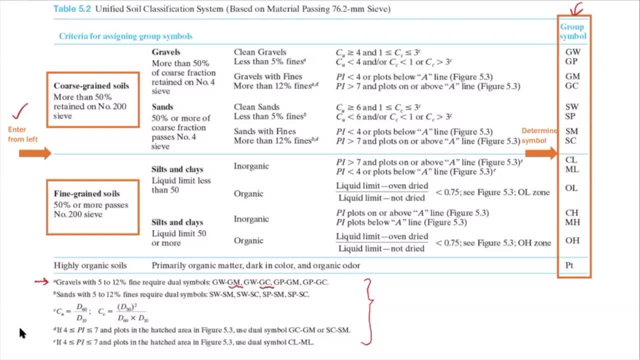 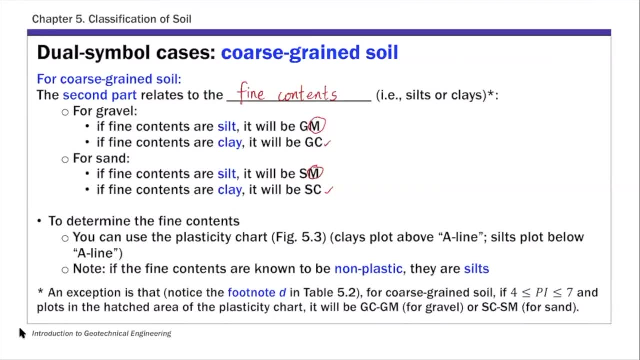 or GC, depending on the fine contents. And to decide which fine contents are in the soil you need plasticity chart. So this is something we covered in the last lecture. If the soil plots above A-line, the fine contents are clays. 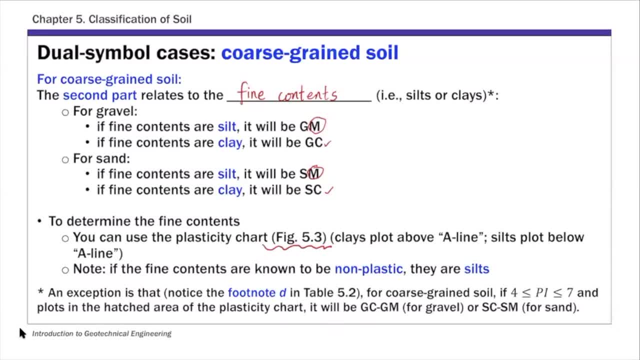 If the soil is plotted below, the fine contents are seals. So that's the plasticity chart. And one additional note I added here: if you know, the fine contents are non-plastic. if it's not plastic, then they're going to be seals. 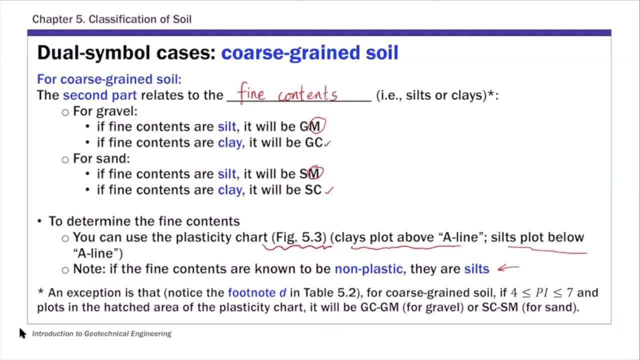 So seals are fine particles without any plasticity. So if you know it's non-plastic, you know the fine contents are seals. Also, there's one exception. So this is foot node D here. That's why I said dual symbol cases are tricky. 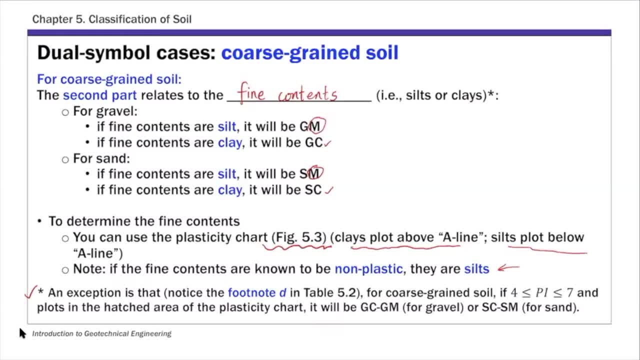 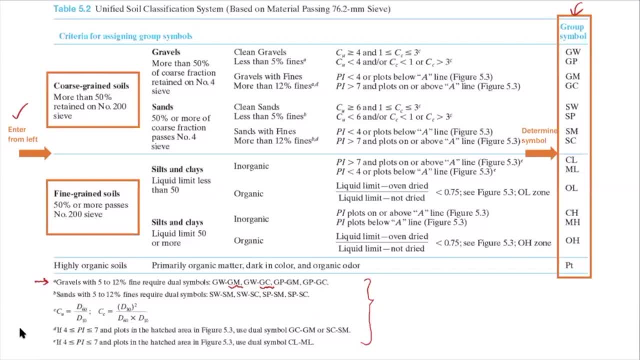 The foot node D here, table 5.2.. So this one here. Okay. So for foot node D, if PI plastic index is between 4 and 7, and plots in the hatched area of the plasticity chart, 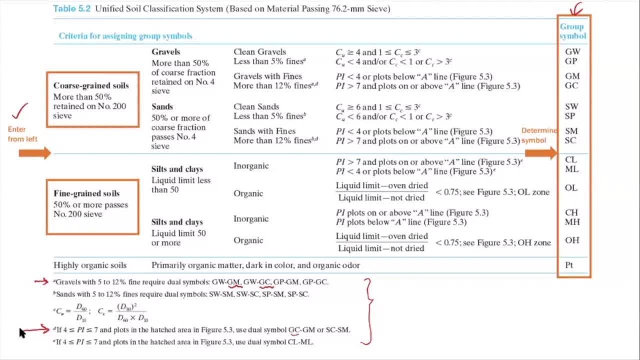 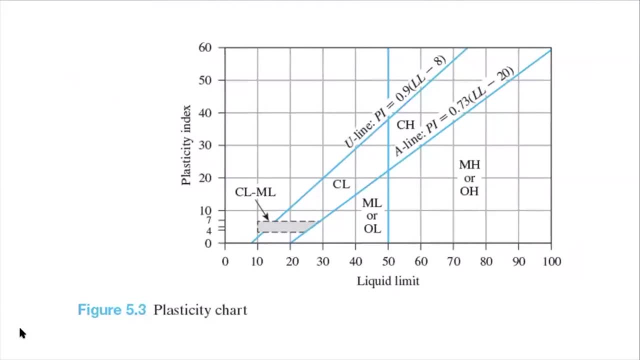 then the dual symbol case would be GC-GM or SC-SM. Okay, So if you look at plasticity chart, so this is the hatched area. So if your PI is between 4 and 7, and it plots in this hatched area, 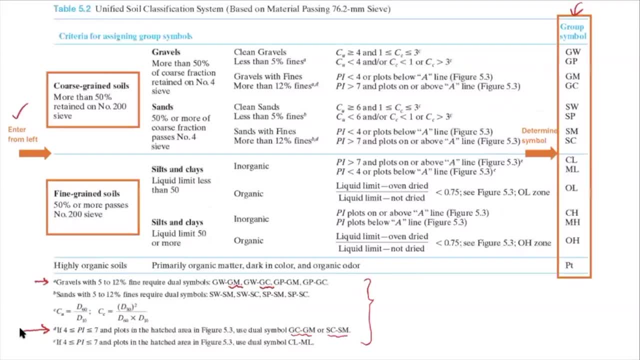 it's going to be either GM-GC, So that's if your coarse grain soil, your coarse components are gravels, or SC-SM, if your coarse grain components are sands, So that's a special case, And then for fine grain soil. 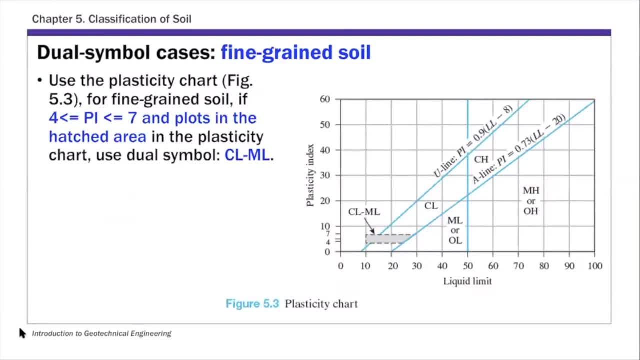 this is simpler than the coarse grain case. Dual symbol cases for fine grain soil is actually pretty straightforward, Just using the plasticity chart. So use plasticity chart if PI between 4 and 7, and plots in a hatched area in the plasticity chart.